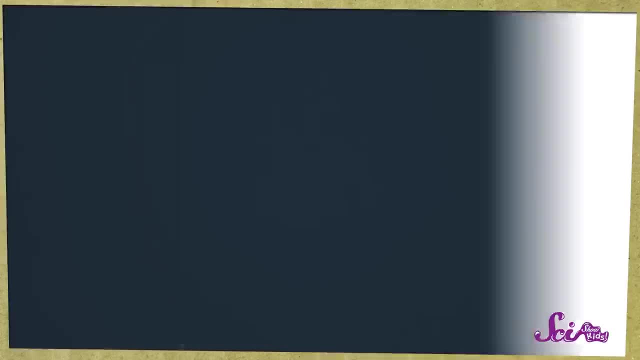 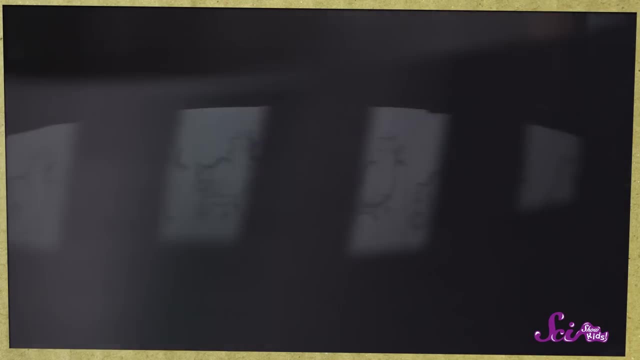 It will be like we're seeing each drawing on its own, but super, duper fast. And then, when we spin the zoetrope, our brains will stop noticing the black space and connect the drawings together. The faster the zoetrope spins, the smoother the animation will be. 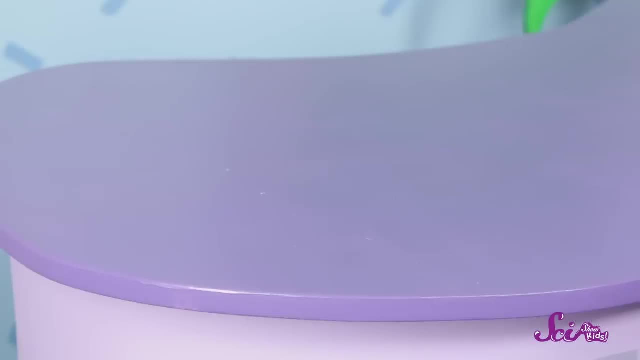 You can make your own zoetrope along with us. All you need is some black construction paper, some white construction paper, scissors, tape, a ruler, two pencils and a pen, And then you're done. We're going to need two pencils, a round piece of cardboard or a paper plate about. 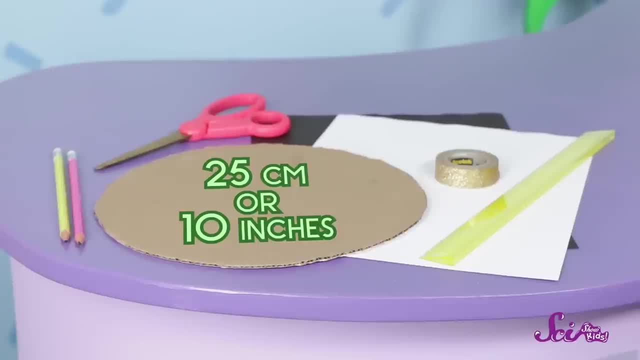 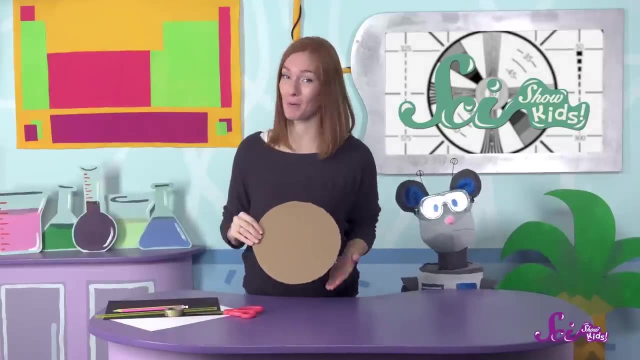 25 centimeters across and a grown-up. to help, because we'll be doing some measuring and cutting For our base, we cut out this round piece of cardboard- although you can use a paper plate. We'll make a small hole in the middle, just big enough to push one of the pencils through. 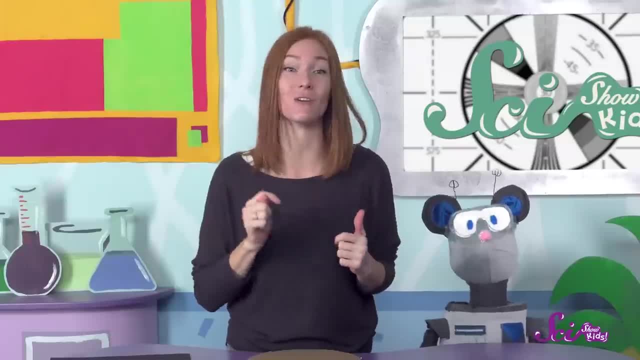 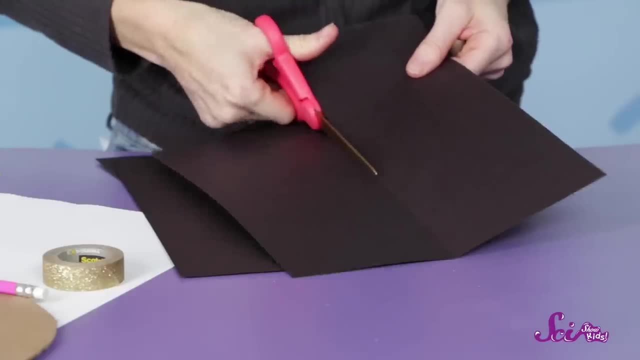 and have the eraser catch on the top, but we won't put the pencil in yet. Next we need to make the walls of the zoetrope. For that we'll use the black and white paper First. we'll cut two pieces of the black paper in half the long way, so we'll have 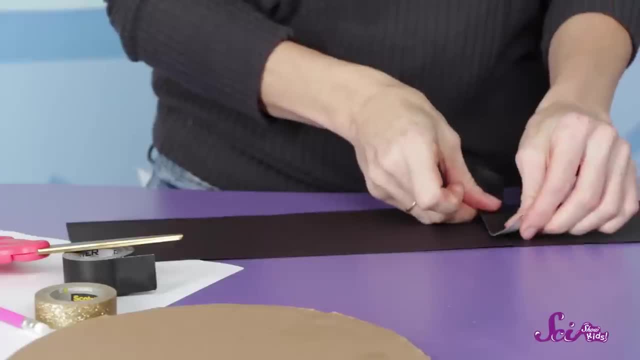 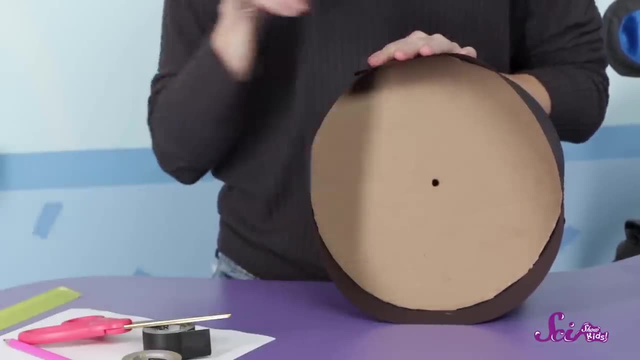 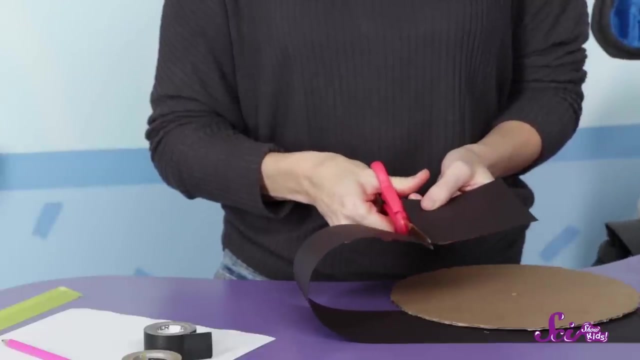 four long strips. Then we'll take three of the strips and tape them together. Next, we'll wrap them around the outside of the cardboard base. We might need to trim a little off the end to make sure it fits exactly. This is where we're going to put the slits. to look through and see the animation. 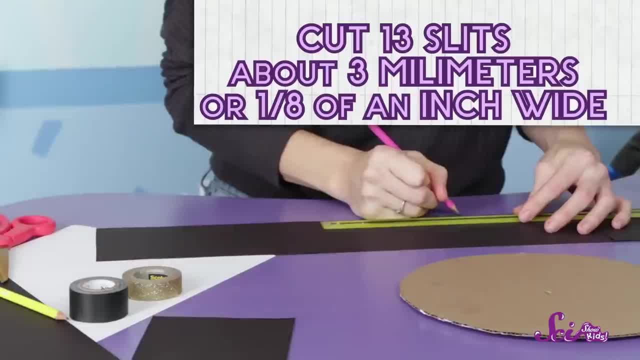 We'll cut 13 slits, each about three meters long. We'll cut them in half. Then we'll cut two pieces of the black paper in half the long way. We'll tape them about three millimeters or an eighth of an inch wide into the top. 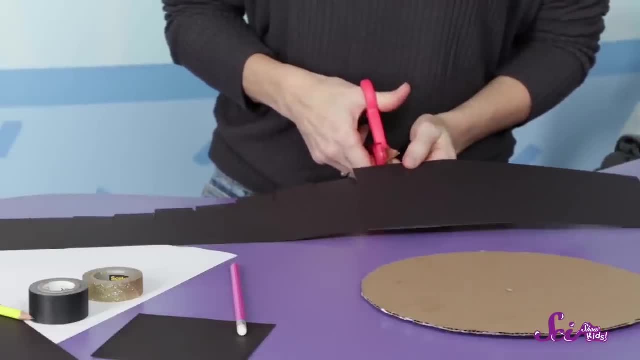 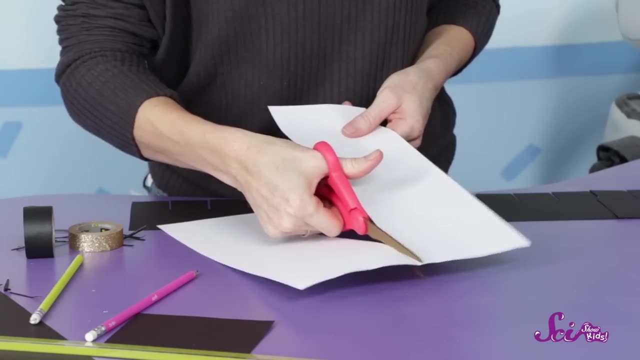 half of the black strip. We'll try to make them evenly spaced, about four centimeters or one and a half inches apart. Just like we did with the black paper, we'll cut a piece of white paper in half, so we have two long strips. 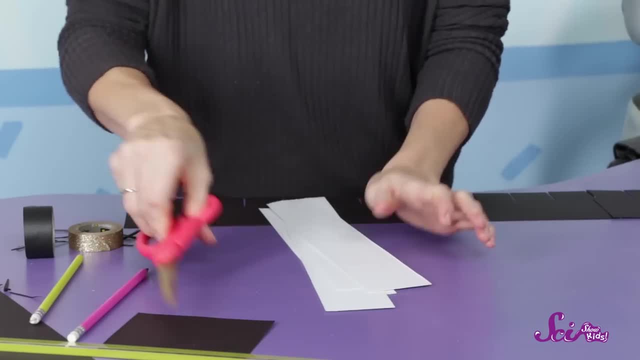 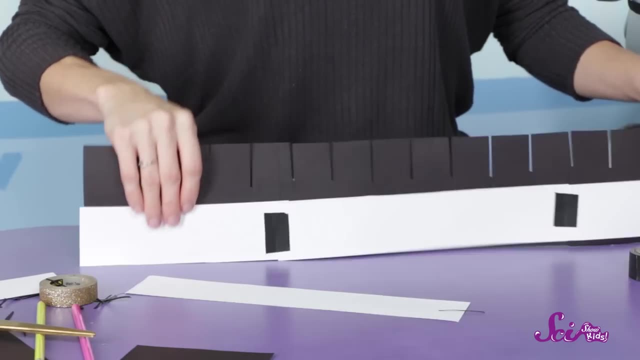 We're going to take those two and cut them in half. That gives us four long strips of paper. We're going to take three of them and tape them all together. Our white strip is now half as tall as our black strip and we're going to cut it so. 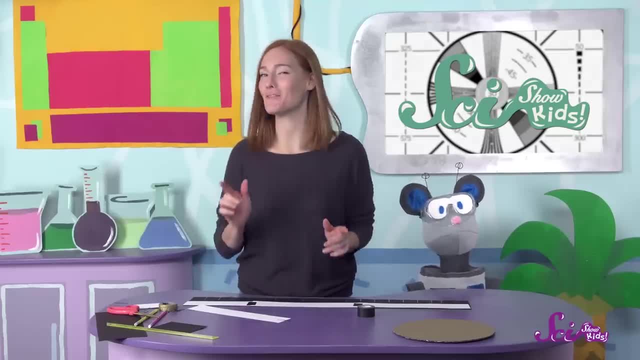 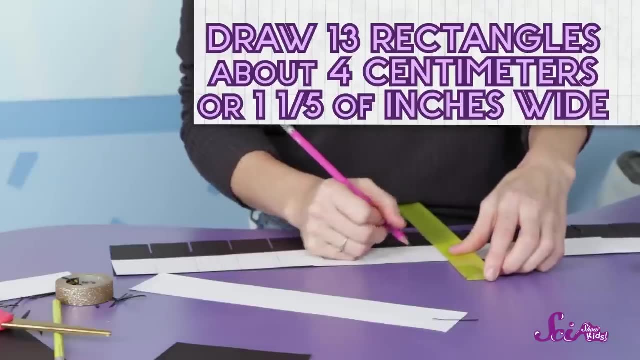 it's the same length. The black paper will become the rectangles we use for each drawing. To make those rectangles, we'll use the ruler and one of the pencils to measure the strips into 13 rectangles that are each about four centimeters or one and a half inches. 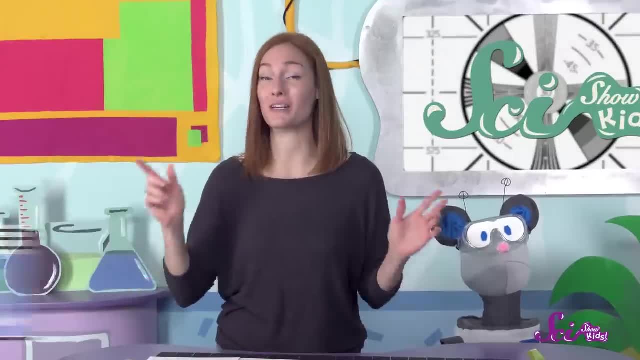 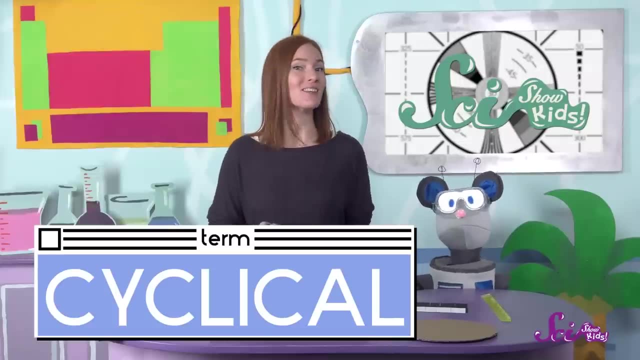 across And now it's time to draw. Our animation is going to be cyclical, which means that as soon as it's done, it's going to start over again from the beginning, So it's good to have an animation that ends right back where it started, like a plane. 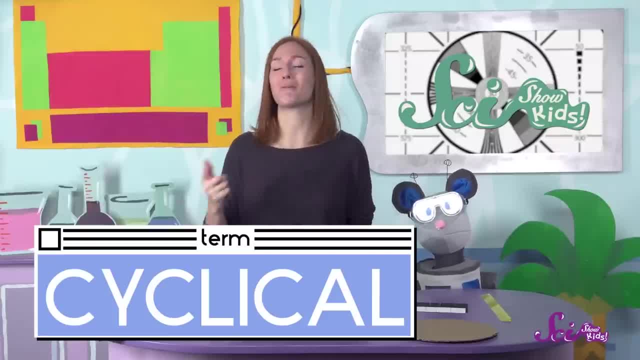 taking off and coming back down, or a person taking off their hat and putting it back on. We're going to use the ruler and one of the pencils to measure the strips into thirteen rectangles that are each about four centimeters or one and a half inches across. 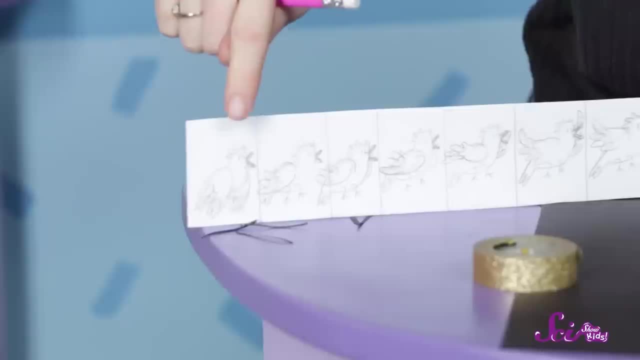 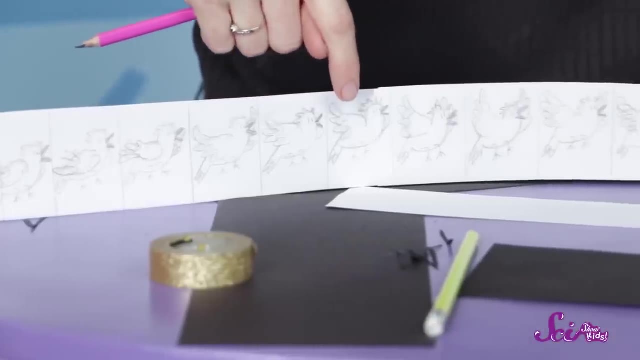 We're going to draw our friend Dino flapping his wings. Each of your frames should look a lot like the last one, with tiny changes from one to the next. See how his wings move up and down, just a tiny bit each rectangle. 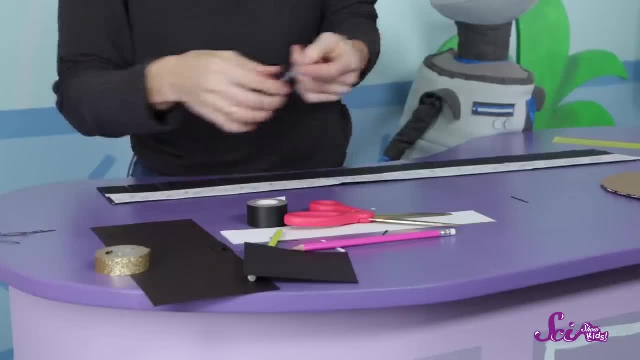 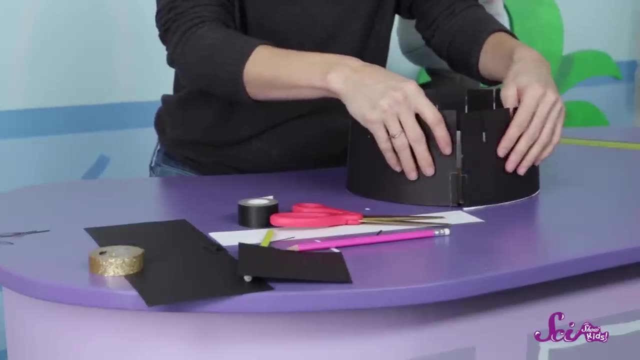 That will help the animation look smoother. Once our drawings are done, we'll tape them to the bottom half of the black paper, with each rectangle right below one of the slits, And now we just need to tape the paper around the base with the drawings on the inside. 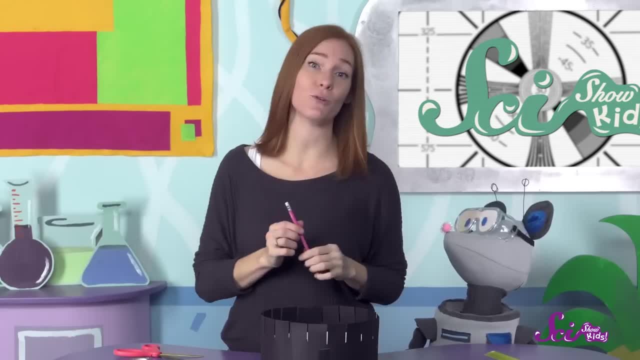 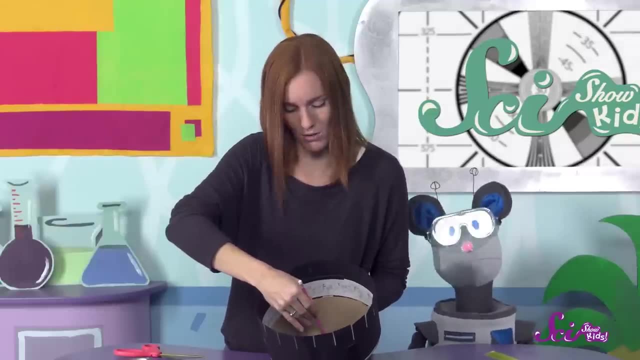 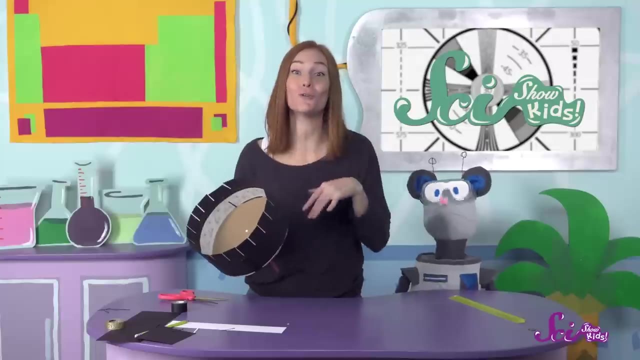 Now all we need is to make it spin. We just stick this pencil through the hole we made in the base earlier, so the eraser catches on the frame and the pencil doesn't fall all the way through. Nice, You could also use chopsticks for this, or glue the hole in your base to a marble. so 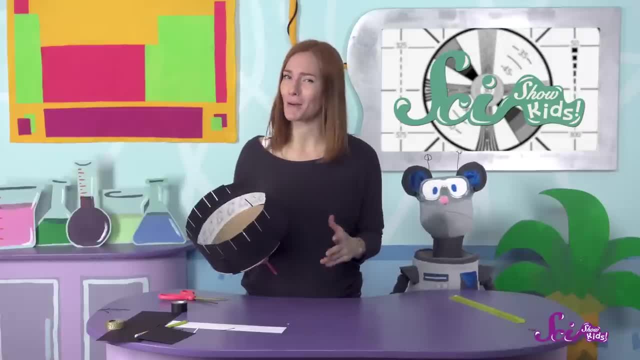 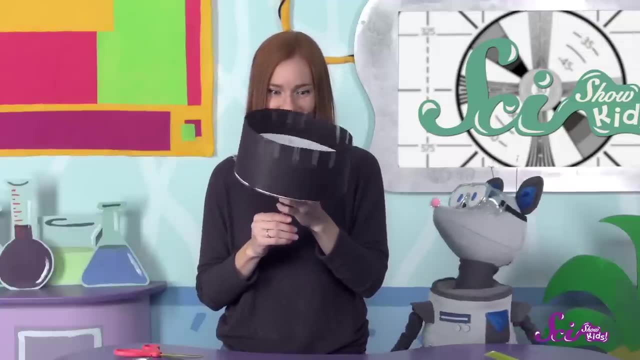 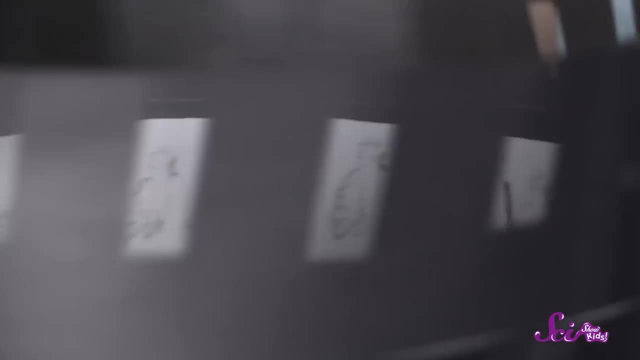 that it can spin on a table. Or, with some help from a grown-up, you might be able to use a record player or a spinning cake platform. And now we spin. Oh cool, Check it out. If the drawings move fast enough, two illusions happen to make them into an animation. 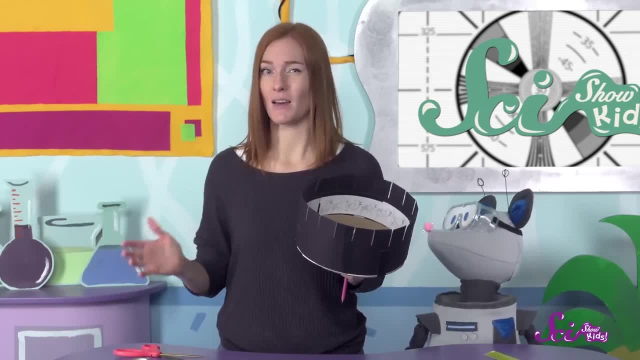 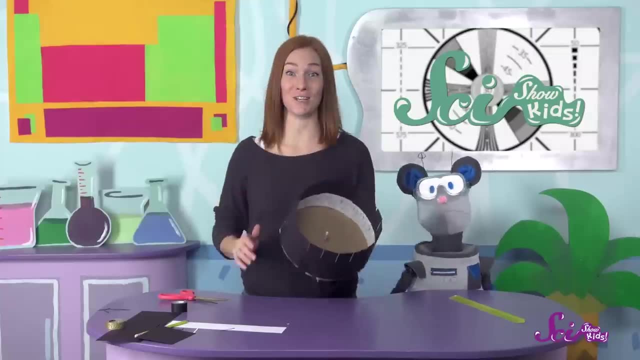 In between each frame there's a blank spot where there's nothing to see. But when the drawings come quickly enough, one after the next, your brain stops noticing the blank spots in between. That's the first illusion. The effect of one picture on your eye lasts until the next one comes up. 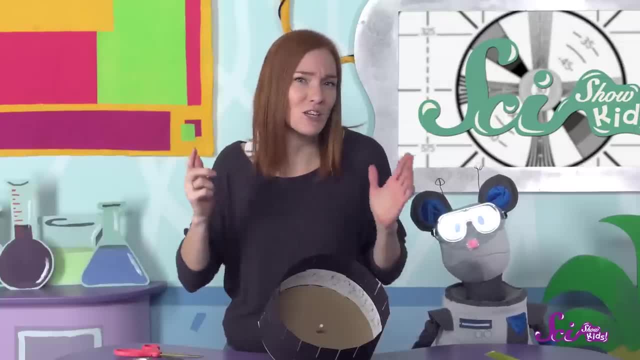 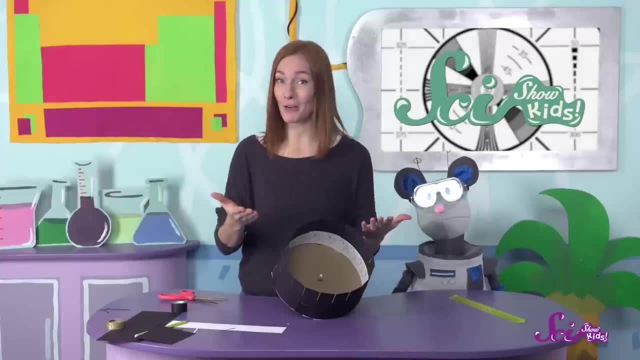 All your brain notices is the drawings. The second illusion is when your brain sees all those separate drawings and thinks that the pictures are moving. It fills in the blanks in between the frames for you and turns them into something that makes sense, like Dino flying. 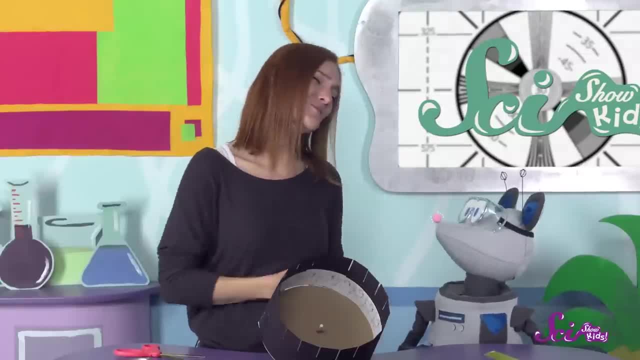 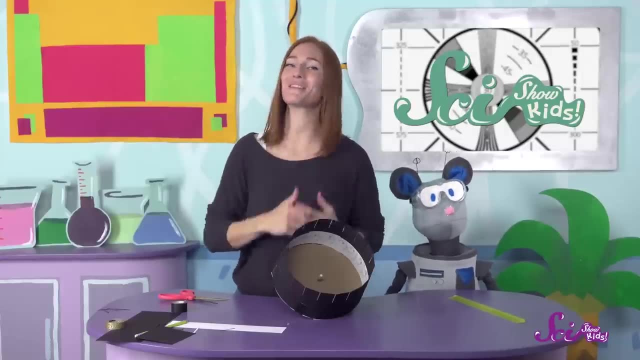 So you can just see the animation and enjoy the cartoon Squeaks. we make an awesome animation team. Did you make a zoetrope too? What would you want to make a cartoon about? We'd love to hear about it.